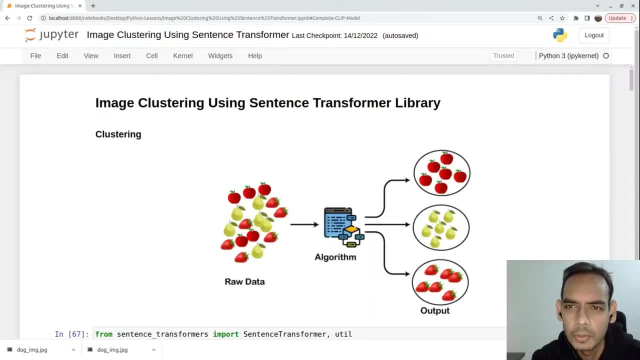 Hey everyone, this is Mayur. Welcome to MLWorks. In this video we'll talk about image clustering using sentence transformer library. So, before jumping to image clustering, what is clustering? Clustering is nothing but an unsupervised learning technique to group a bunch of records which are 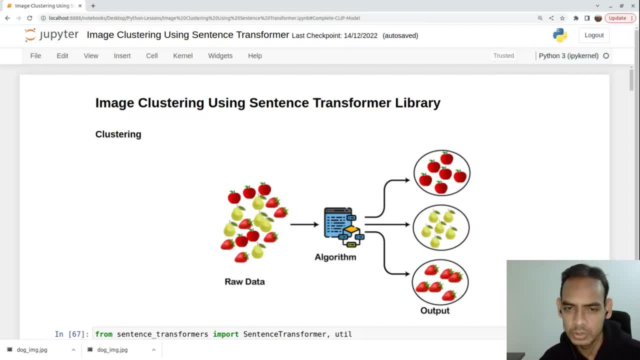 similar in nature. For example, if you have a raw data set of fruits, each fruit has its set of color, shape and other distinct patterns on it. The algorithm tries to identify those patterns and group them together to form a cluster of that particular object. So basically, 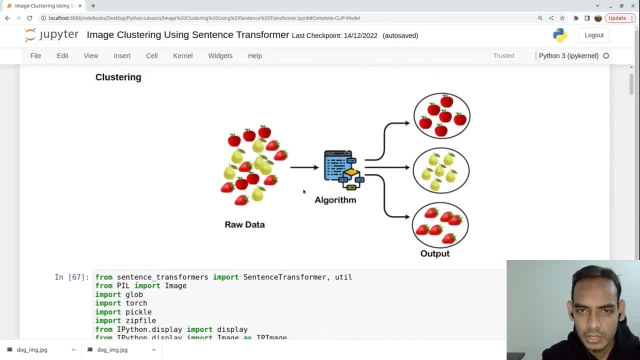 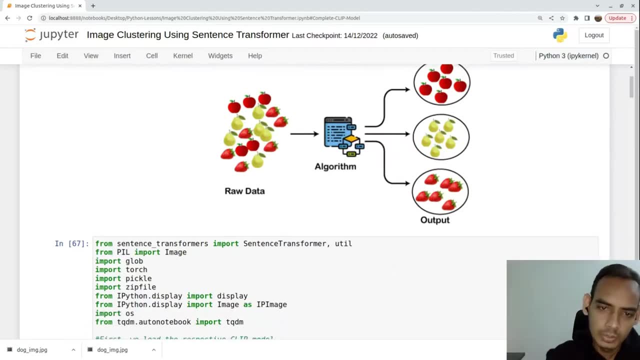 that is a simple definition of clustering And for image clustering, what we'll do is we use a sentence transformer library which has many pre-trained models, And for this exercise we'll be using clip-based model, which is nothing but contrastive language image pre-training. 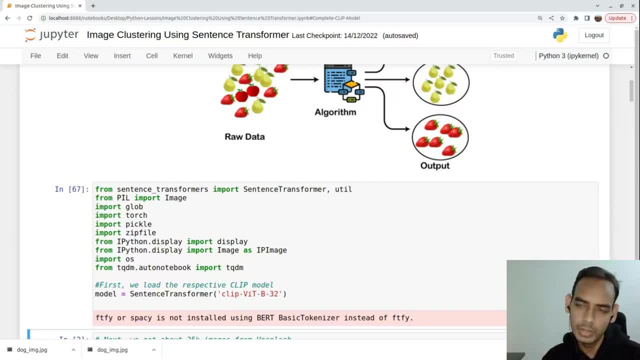 which is trained on a data set which is containing both image and text corresponding to that particular image. So it has been trained on that. So what we'll do is we don't need the end goal of this particular model, which is like generating an image. 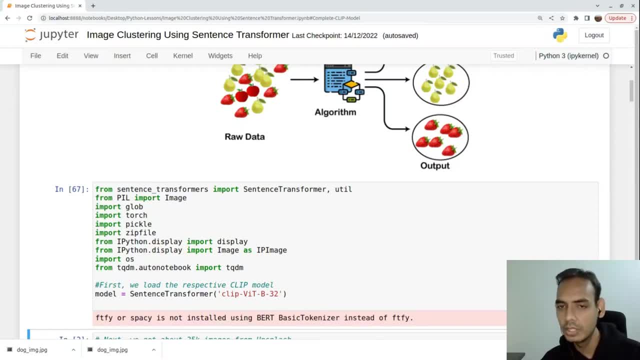 based on the text. So what we do is we just need the image aspect of it. since we are using this image clustering right, What we'll do is we'll just take an image, we use the image encoder aspect of clip model and generate the embeddings. So in sentence transformer we directly have what 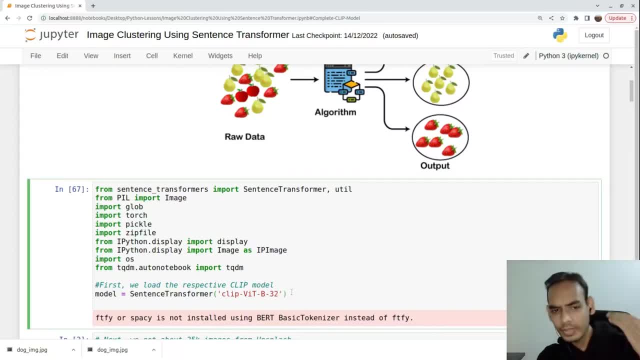 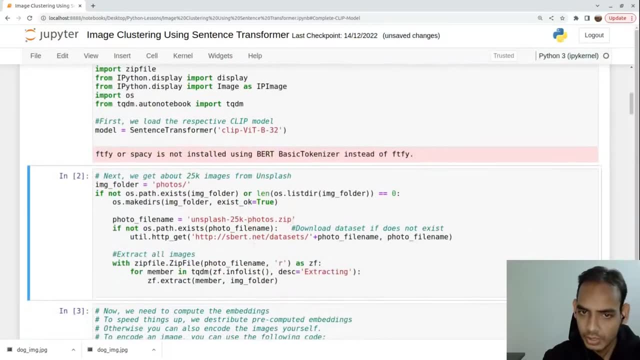 models like clip PIT B32. We just load those models here And we also have a data set of unsplashed 25,000 images And we'll load that as well And totally, there are 25,000,. 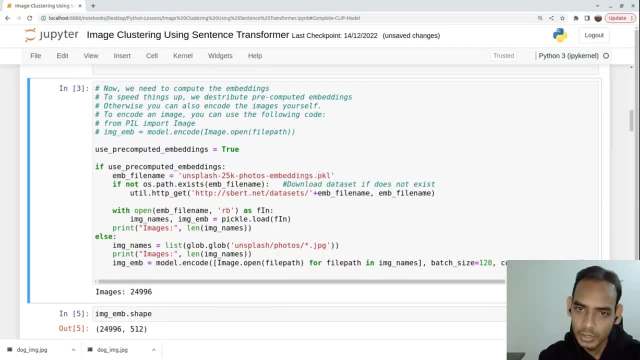 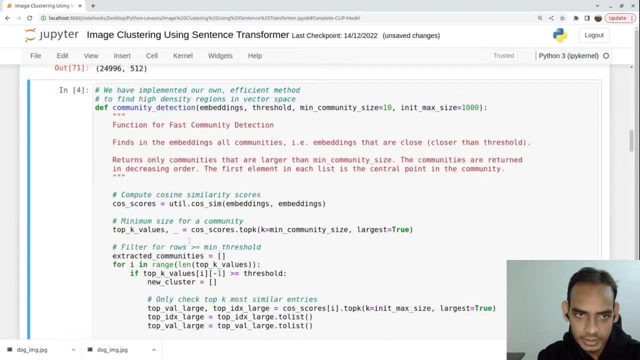 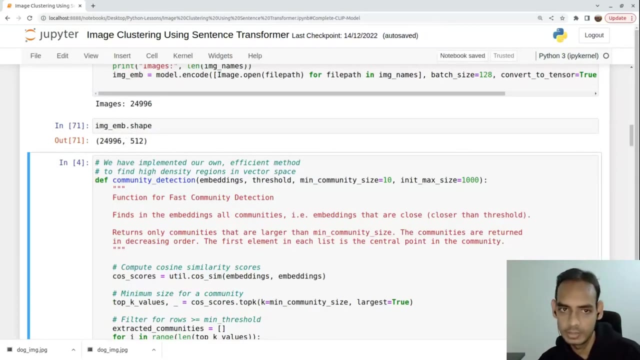 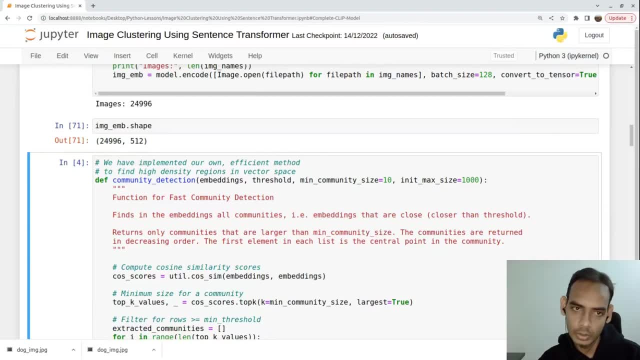 So if you have an image of what 700 into 712. It will be turned into a vector or a list of numbers of 512, of length 512.. Okay, that's what it means. So you have like for 25,000 images. 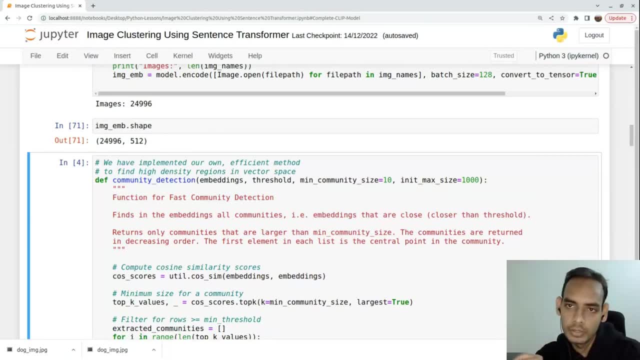 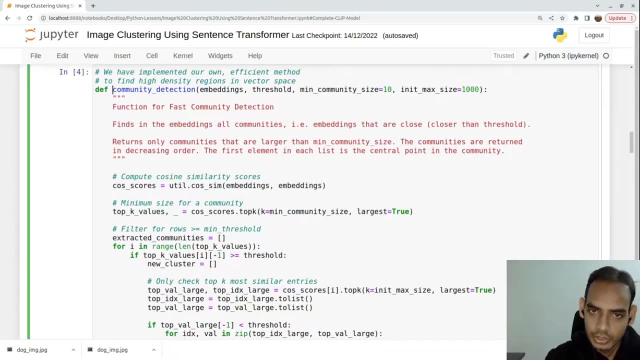 per image you have 512, list of number representing that particular image. So next, what we do is we have, we write a community detection function. what it will do is it will generate clusters based on the images. Now how you want your cluster to be. 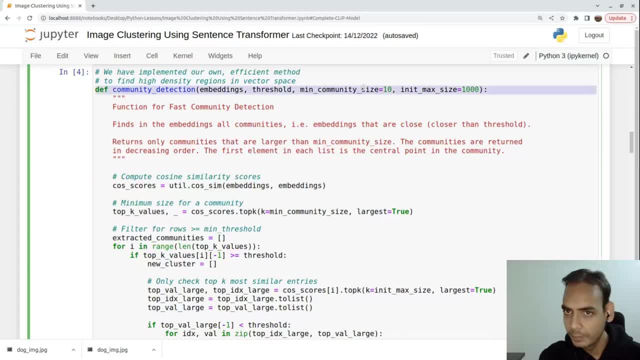 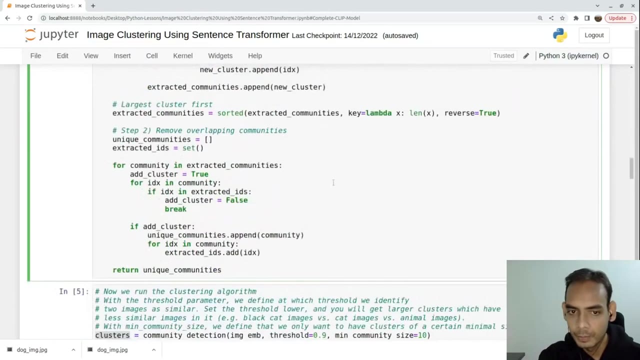 so per cluster we need a minimum community size of 10.. That should be at least 10 images per cluster And the threshold is that each inside those cluster the record should match about 90%, Because threshold is what we give here while creating those community right. 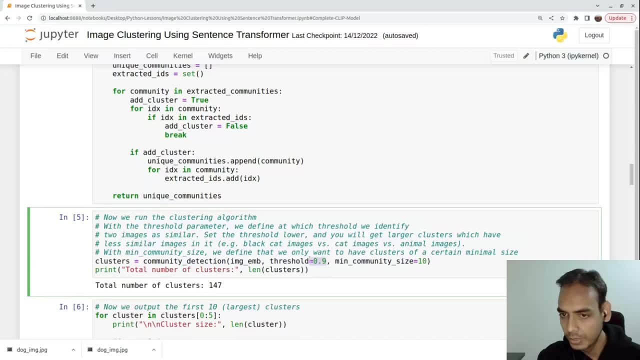 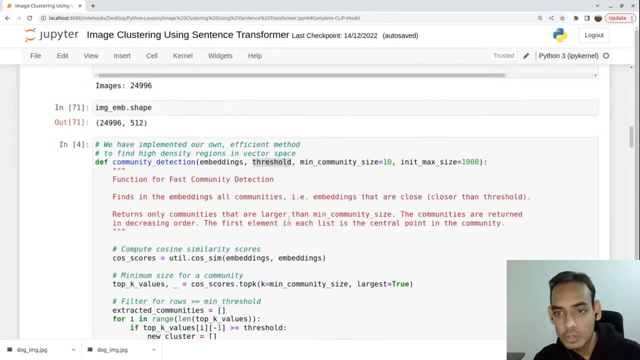 it should match at least 90 percentage of similarity should be there. the cluster should happen. So these are some some of the parameters we're passing here And we are also passing the init max size. there should be at max you can have only what. 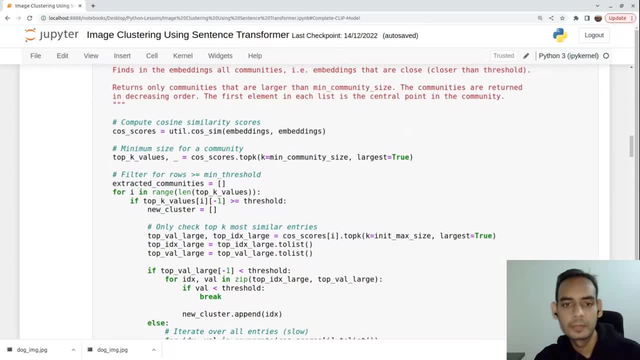 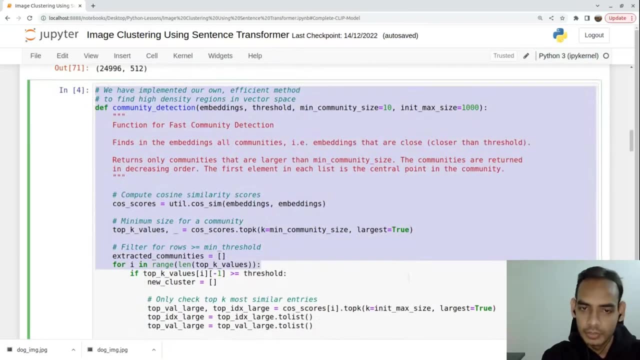 1000 images inside one cluster, So this is not a very big deal here actually, with respect to what the kind of thing we want to achieve. This is just what we do is we compare, generate an embeddings, we find the cos cosine similarity. 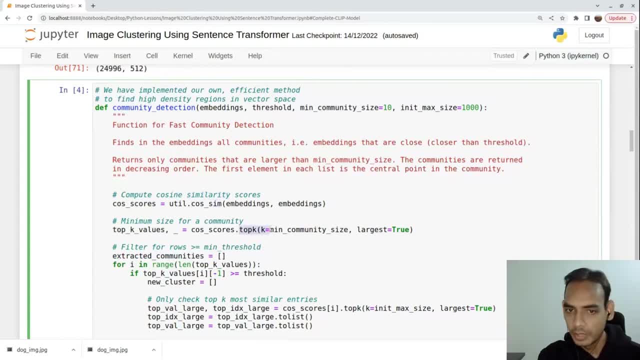 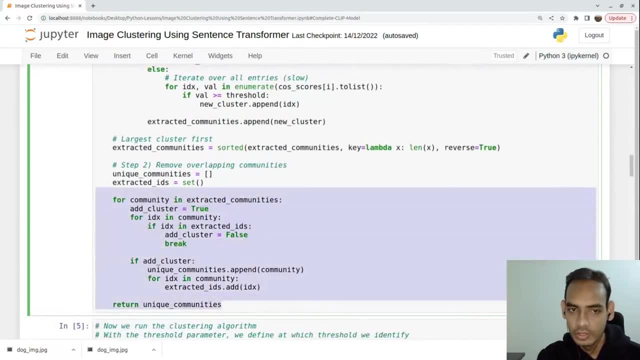 score and on the top of that we find out the top k, which are similar to each other, and we create a bunch of clusters and also what. we also make sure that one image is not present inside multiple clusters. So we create unique communities and what we do is, if the already a particular index or 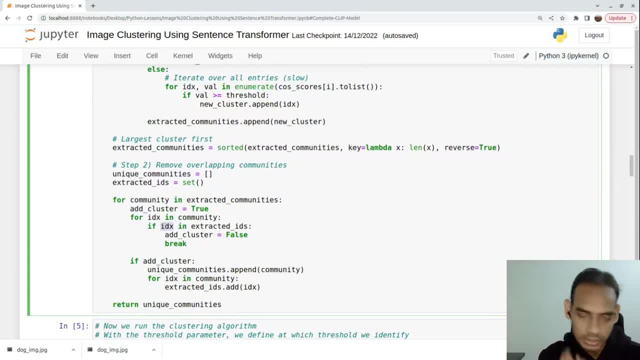 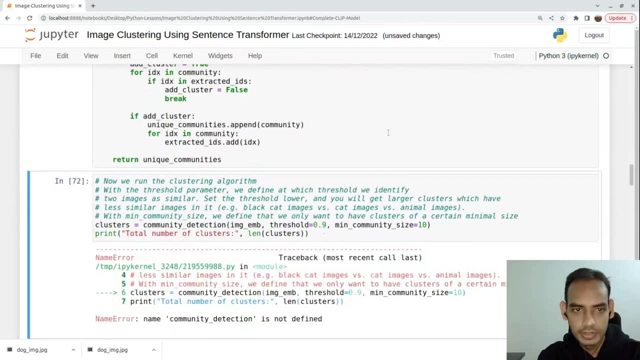 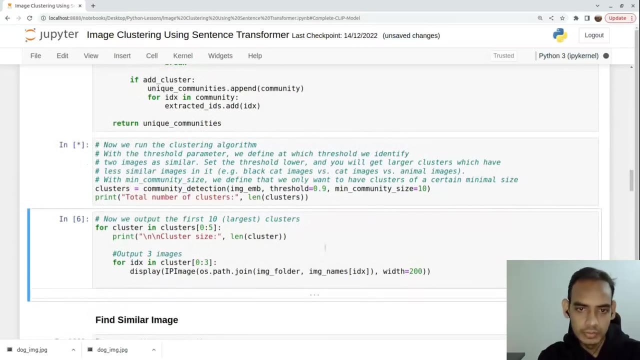 particular image is already present in one community, it should not be present in another cluster or another community. So let's define that and run this total number of clusters So it will generate a number of clusters. It will generate around 140, some clusters we have. 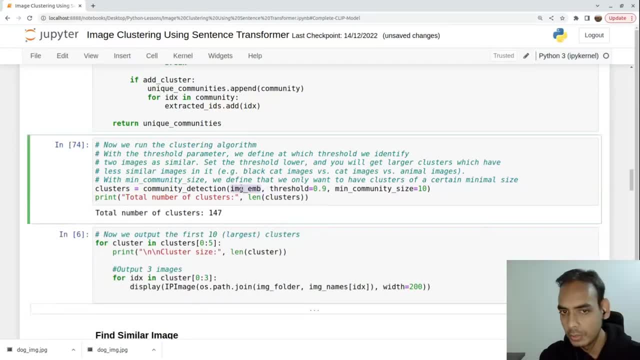 If you see here, what I am passing is I am passing all the 25000 images inside it and then clustering all the records and creating these communities or clusters, and it has this constraints, like it should. while you are creating the clusters, the images should have a similarity of around. 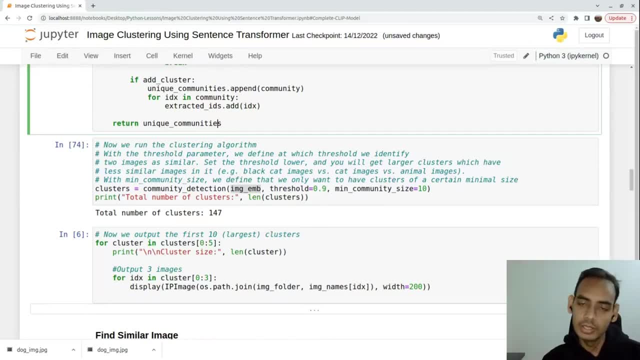 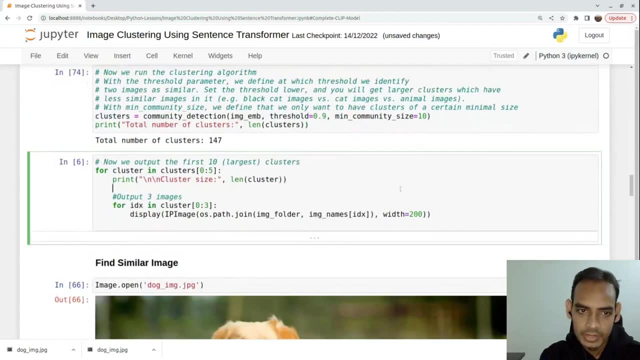 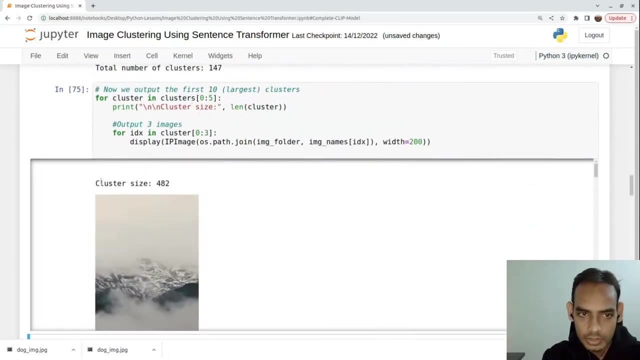 90% and there must be at least 10%, 10 records per cluster. So at the end we get around 147 clusters And we are just looking at each of those particular clusters here per cluster. how this, for example, cluster size of 482 images. 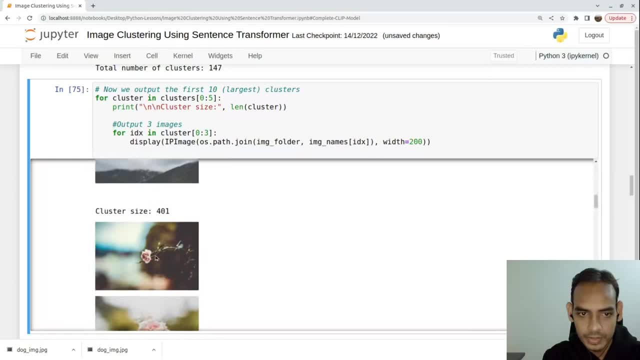 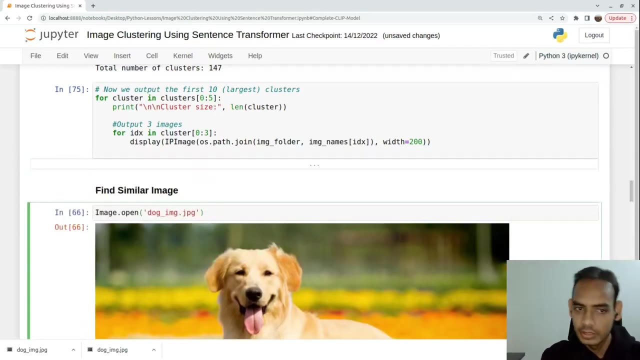 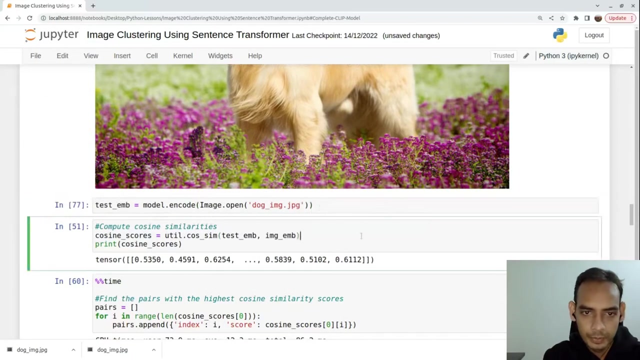 So these images, all these images, are falling under one cluster. Similarly, these 401 images are a cluster of flash. Similarly, this is for an ocean, or whatever. okay, now what I will do is I already downloaded an image from internet Which is a dog's image, okay, and I am creating a test amending of that particular image, okay. 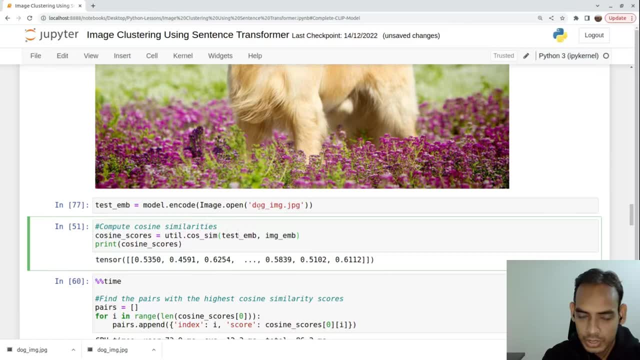 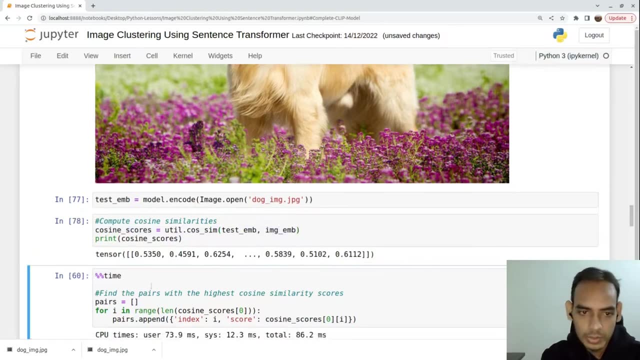 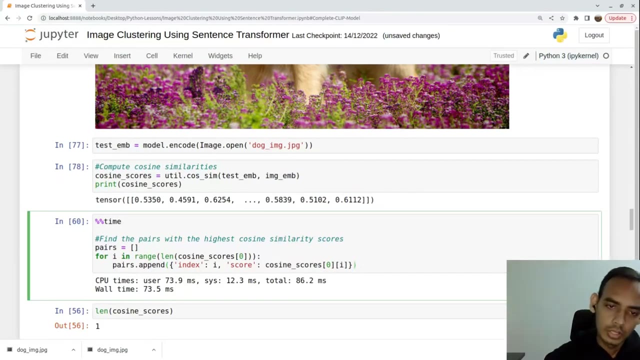 and finding a similarity of this particular image with the 25000 images. we already have image amendings of that, okay, So once we have done that, then we are trying to what map, the index and also the score corresponding to it. okay, Once that is done, 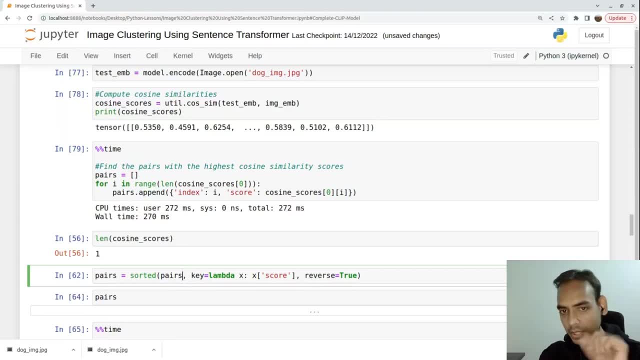 We sort Pairs like index and score pairs based on the highest score of the particular index, For example some images. for example, if you see here at 0 index you have 0.53, and second index you have 0.45 and here we have 0.62, and we sort it in such a fashion that highest 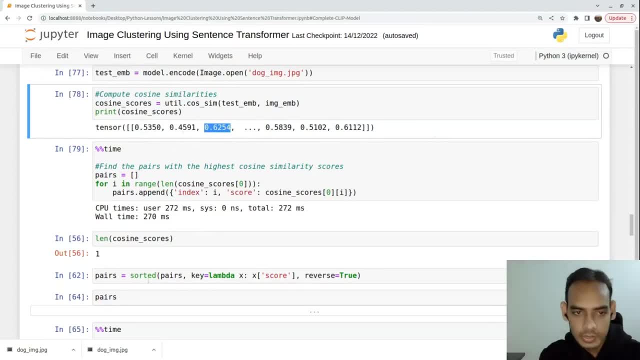 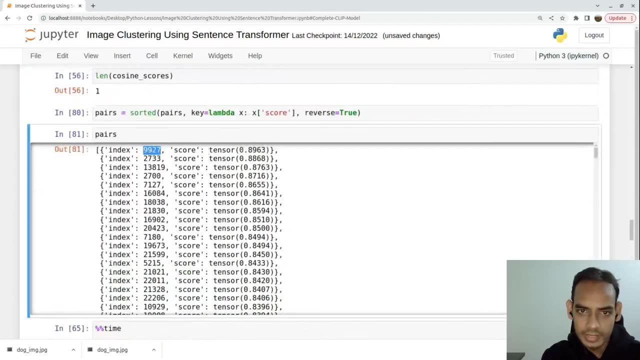 score is at the top and the lowest score is at the bottom. So we will run this and if we see the pairs, we will see index and score. Index and its highest score is 0.89, 27, the index and we say the score of 8868. 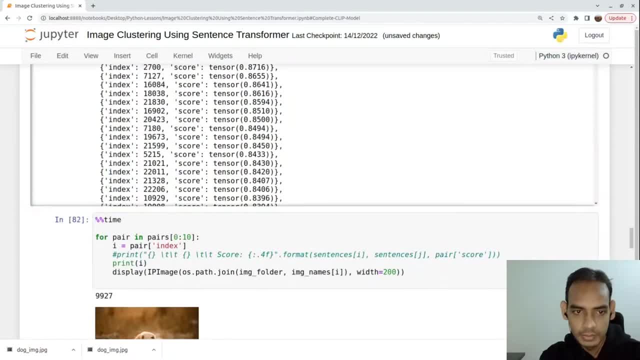 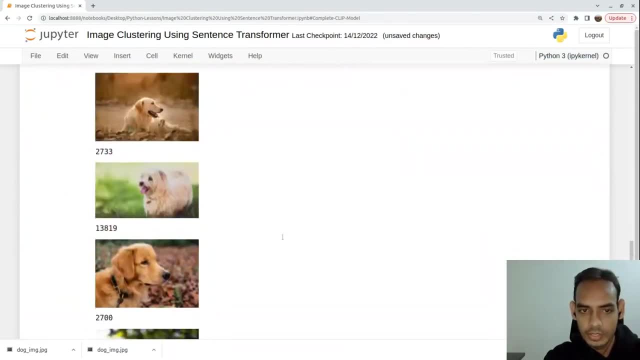 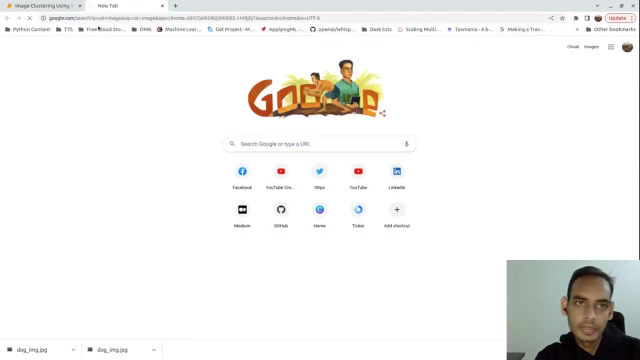 Now we will iterate through these pairs and we will see similar images. This is similar image to this particular dog image. we have corresponding similar images. Now what I will do is I will download an image of cat image and then let's see. Okay, 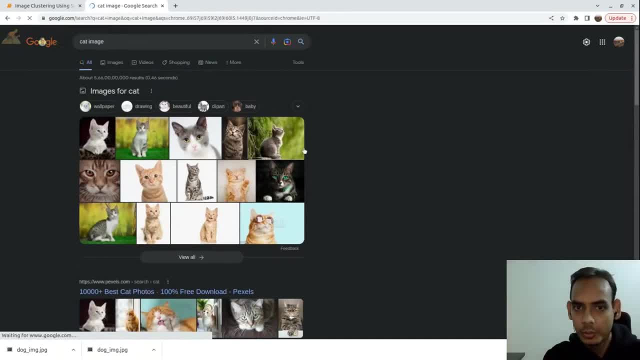 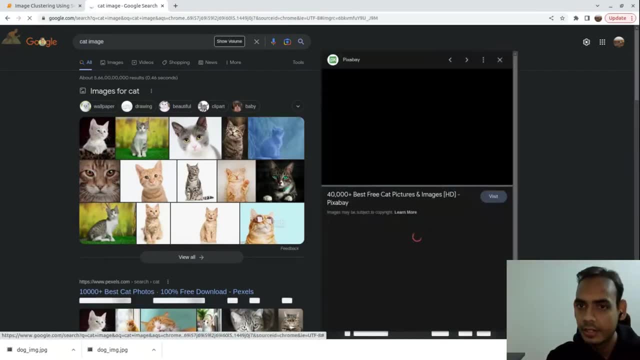 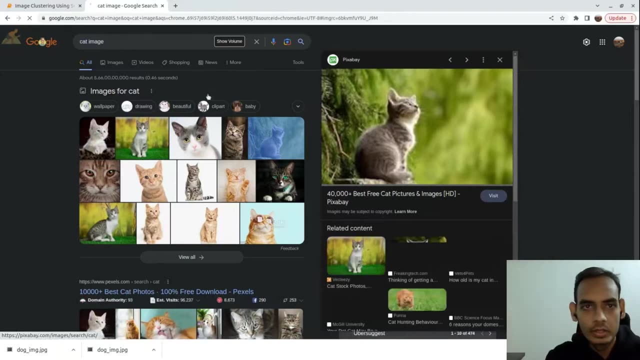 Okay. Okay, So we will generate, download this one and generate an embedding of this particular image, and then we will try to form or find corresponding similar images to this one. Okay, Save this image. Okay, I guess my internet speed is slow. 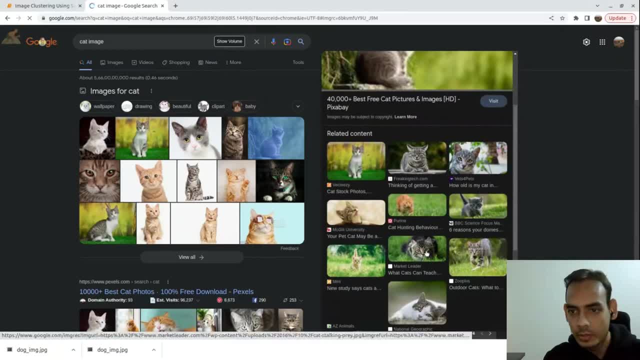 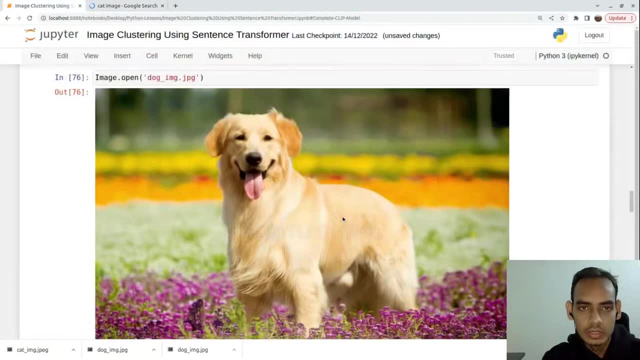 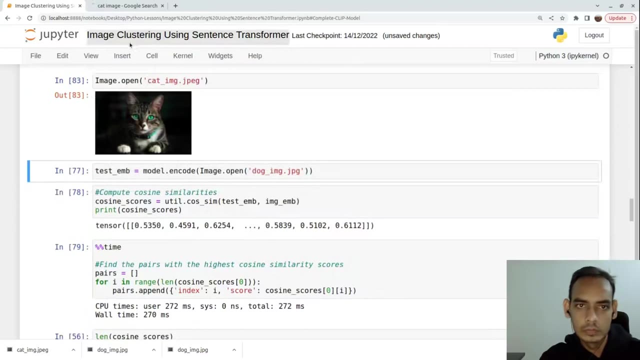 Let's download this image. Save the image. Okay, This is cat underscore image. Let's load that particular image here. Let's see we are able to generate them and this looks like a very small image. Let's see, Okay, Okay.